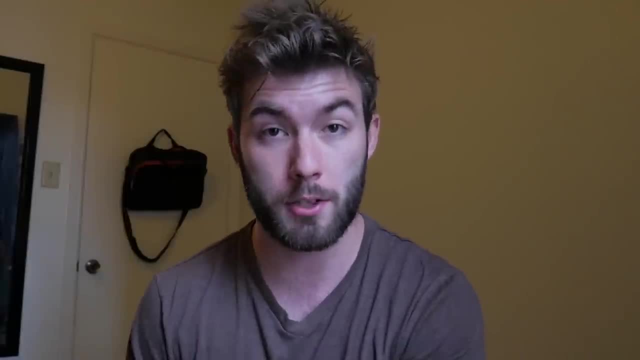 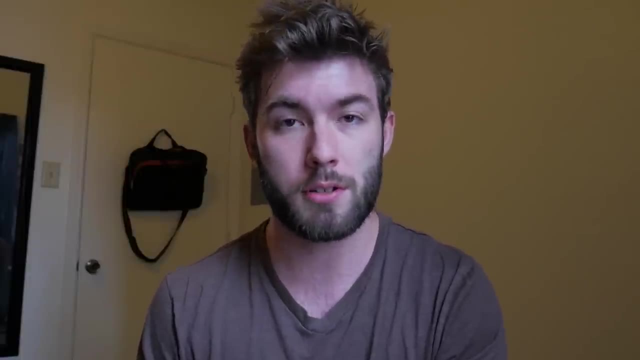 Well, maybe not necessarily complete, but it goes over Lagrangians and Hamiltonians, and it does that for two reasons, The first of which is Hamiltonians are super useful in quantum mechanics because the Schrodinger equation is written in terms of it. 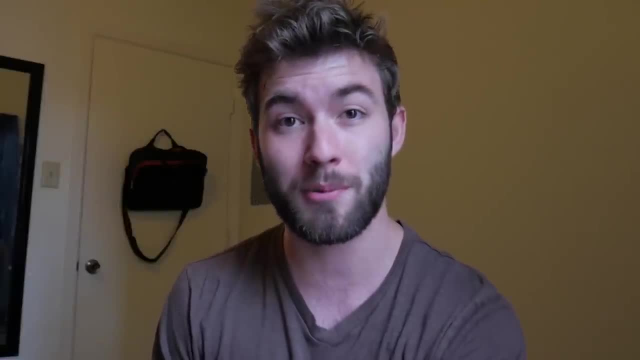 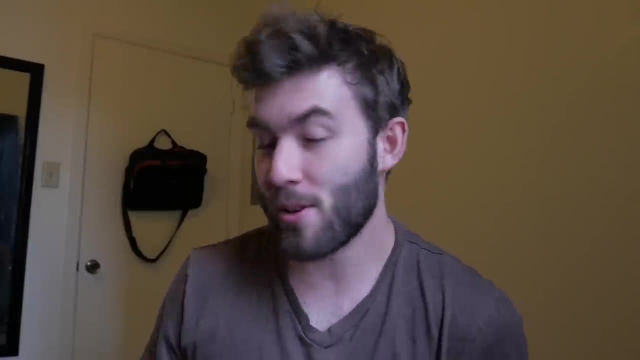 And when it comes to Lagrangians, well, this book also has two chapters dedicated to the path integral formulation, Feynman path integrals, which is where Lagrangians become important again. So so far, I like that this book seems to be a little bit more complex than the other chapters. 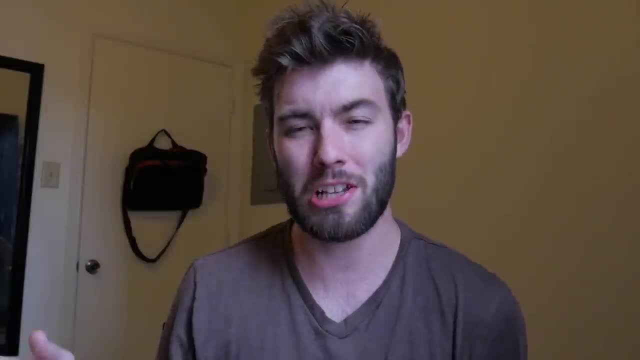 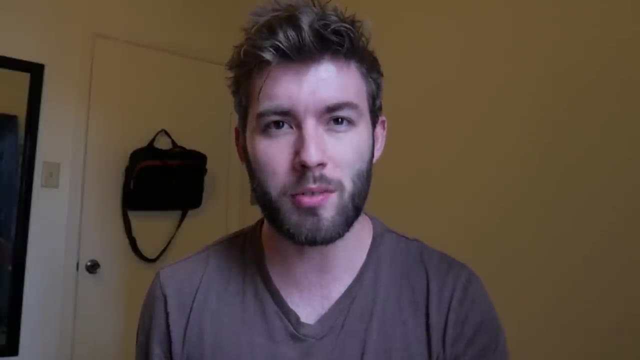 I like that this book seems really thorough, I like that it walks you through the steps and I also really like that it starts right off the bat with Braquette notation, Dirac notation, which Griffiths sort of danced around. He would write a whole bunch of psi-star-sis instead of having like Braquette. 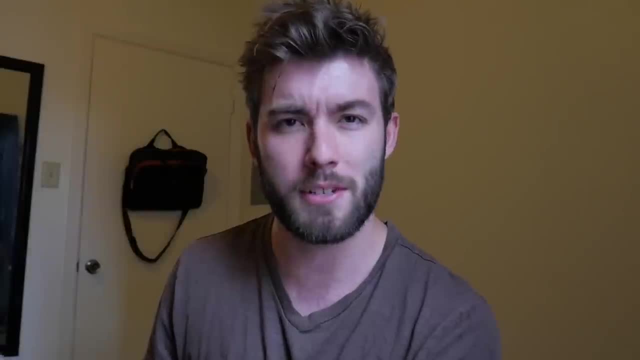 Braquette notation is just, it's so. it's so simple. it's a small part of this book, but it's still something that I enjoy. This book just really seems to go from the ground up, like it starts with math. that's important, so everyone's on the same page. 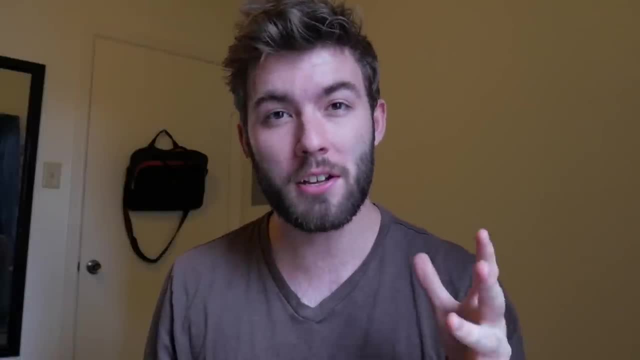 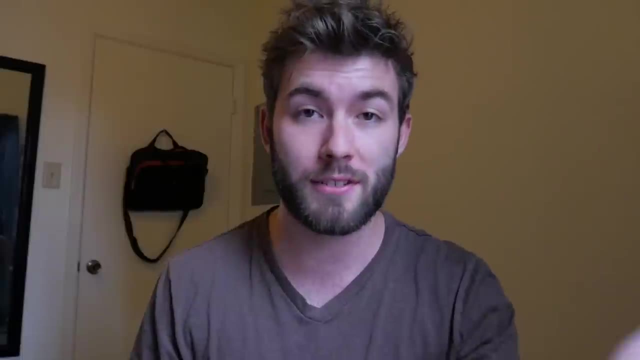 then it goes into classical mechanics, which everyone should really know, and then it goes to where classical mechanics starts to fail. then it goes to quantum mechanics in one dimension, talks about the double slit, probability, uncertainty. then to the Schrödinger equation. 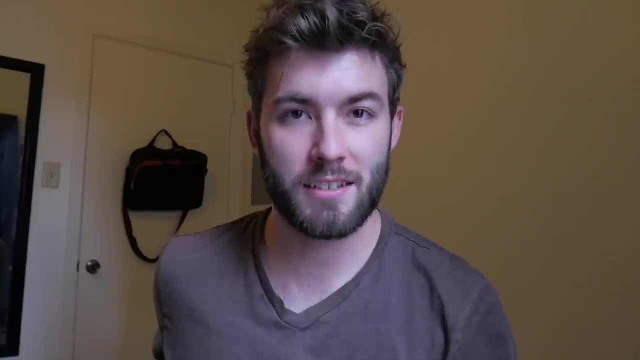 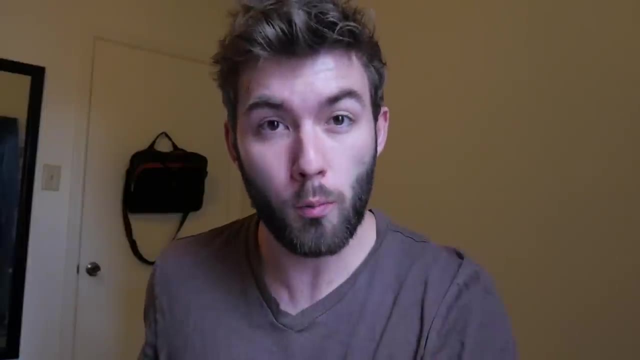 It just. it just seems like it's a good flow. It then gets into more complicated and involved aspects of quantum mechanics like spin, the hydrogen atom approximate methods, and I hope we get to this next thing next semester. We're definitely not going to do it this semester. 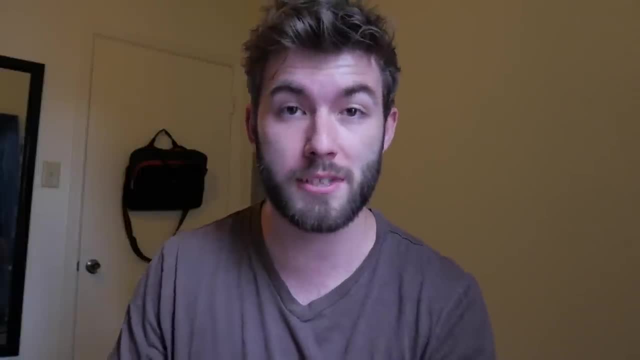 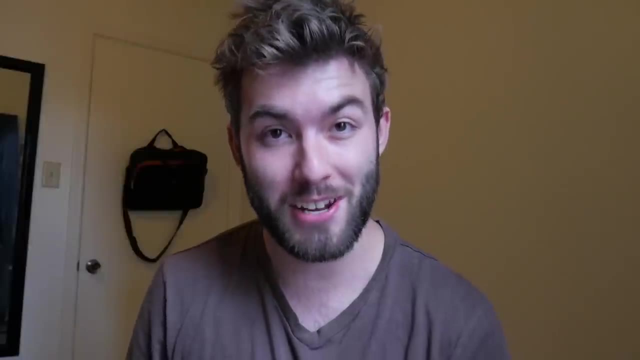 but there's also a section on the Dirac equation so it gets into relativistic quantum mechanics So the material looks fun. The attention to detail that Shankar seems to have in the book I can really appreciate and I hope it carries through with the rest of the chapters. 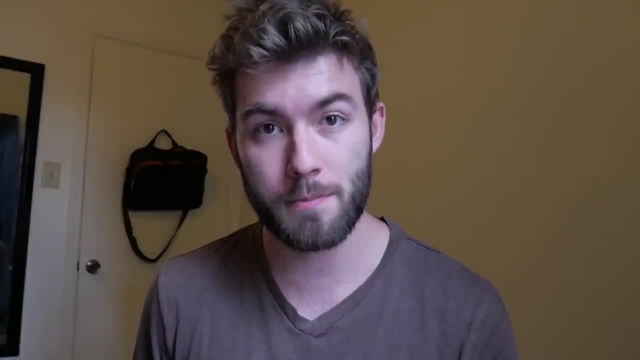 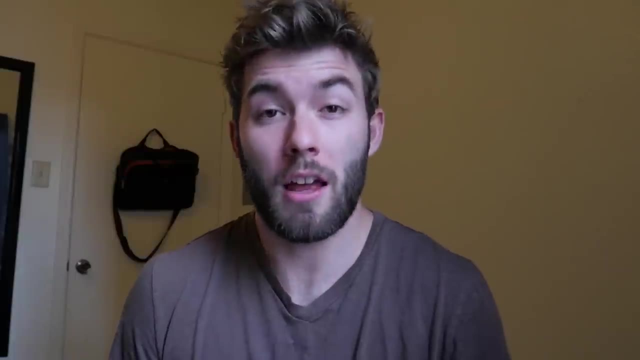 I'm going to leave a link in the description so that you can see the PDF version of this book and let's get started with the next class, which is mathematical methods for physics. I hope I don't spoil this for anybody, but there's a lot of math in physics. 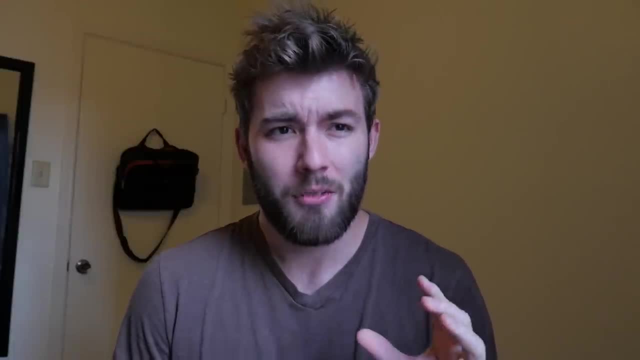 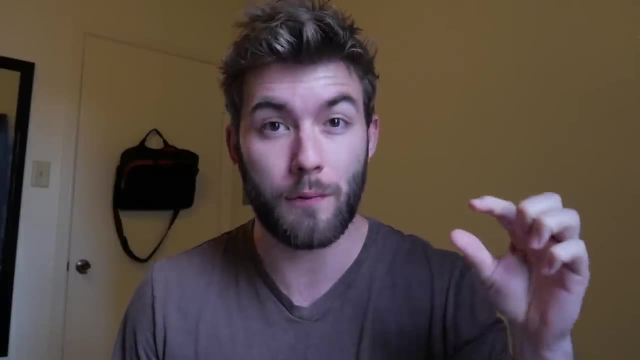 and not only that, but there's a lot of branches of math in physics, and when you're looking for a mathematical physics textbook, I'm not looking for one that tries to condense all of those different branches of math into a 500-page textbook. 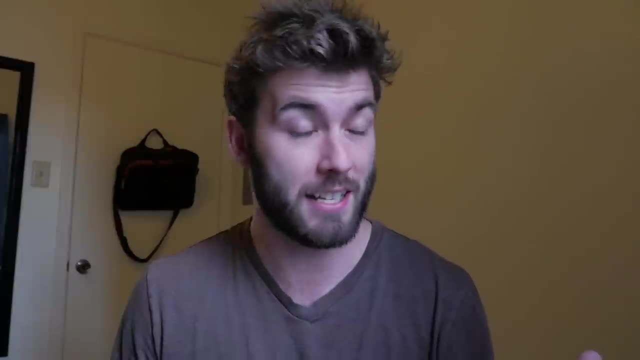 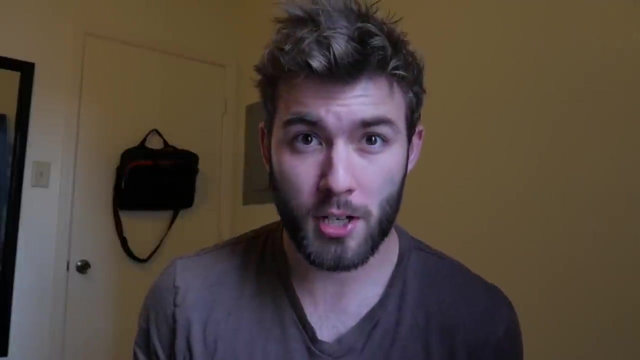 So this book that I'm using now doesn't have 500 pages, It's not 600 pages, It's not 700 pages, It's 1,300 pages of math. I am, of course, talking about Mathematical Methods for Physics and Engineering by Riley, Hobson and Bentz. 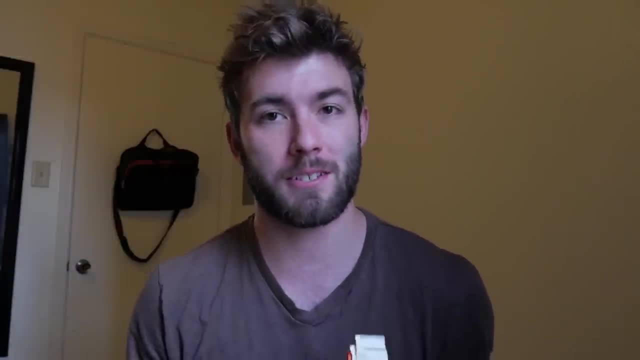 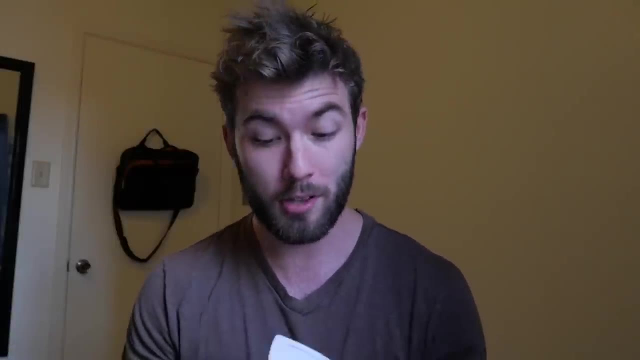 This is probably one of my favorite books that I own simply because it serves as such a good handbook and reference book for math that you already know. I don't really use this as a textbook to learn new math and, believe me, there's plenty of math that I've never even used. 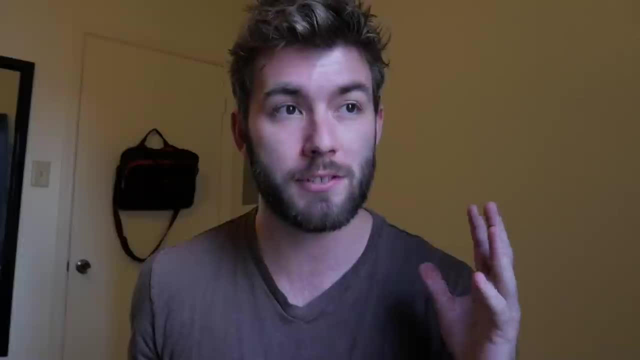 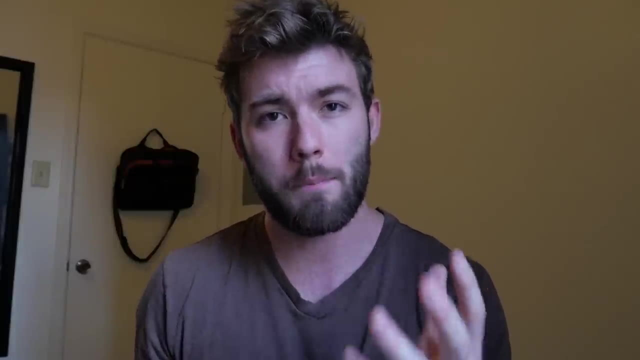 before in this book, but it is a good reference book. If I need to learn something, I'll find a textbook on that branch of math. but one of my favorite things about it is that it's written by physicists for physicists, so there's no theta phi confusion. 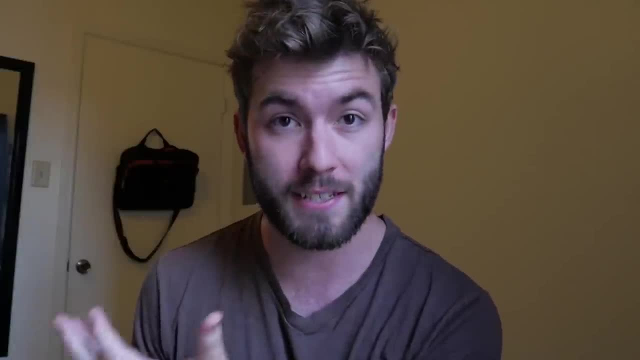 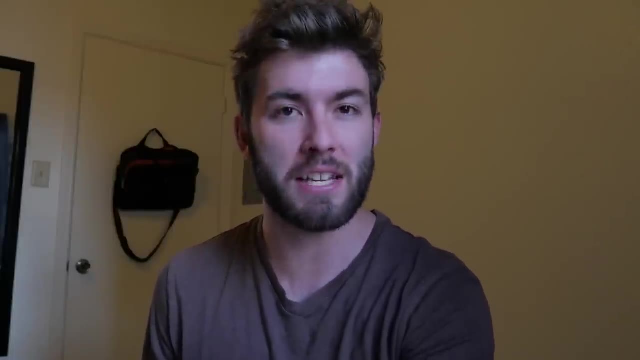 It's all written in the way that you'd be learning it or applying it in your physics classes. Now, though, I don't really typically use this as a textbook for learning new math. you definitely can, and it doesn't really skip many steps or anything like that. 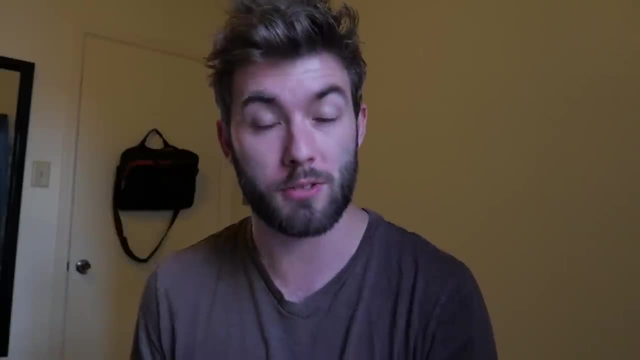 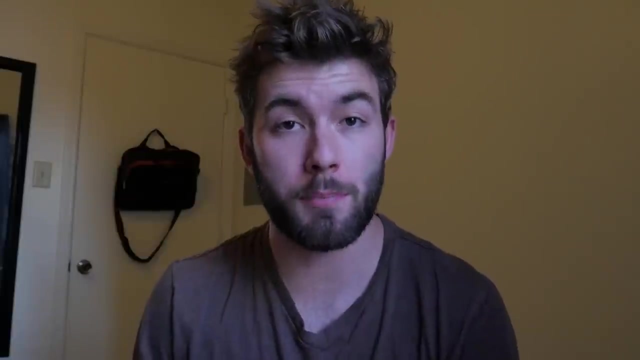 in developing, like the theory of certain theorems. So that's good and that's nothing that you really need to worry about. It's pretty thorough. still, Some of the what I view as important topics that this book goes over is your single and multivariable calculus. 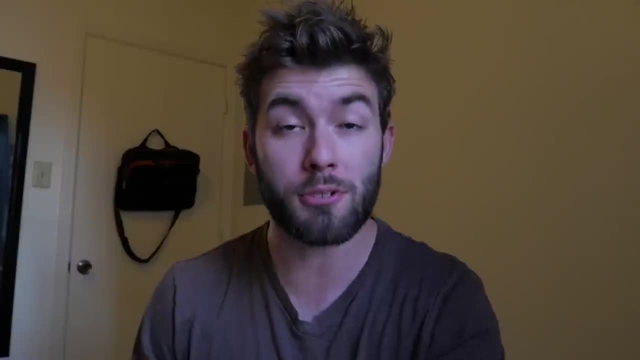 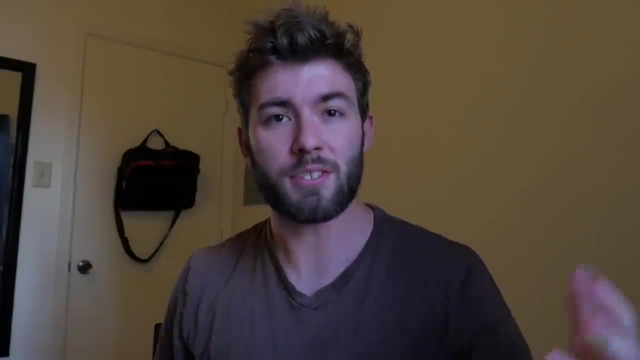 differential equations, vectors, complex variables, partial differential equations, integral transforms, group theory, tensors- I might have already said that I just think tensors are pretty cool. It also goes over statistics, probability and even numerical methods. Overall, I think it is a great book for math that you are fuzzy on. 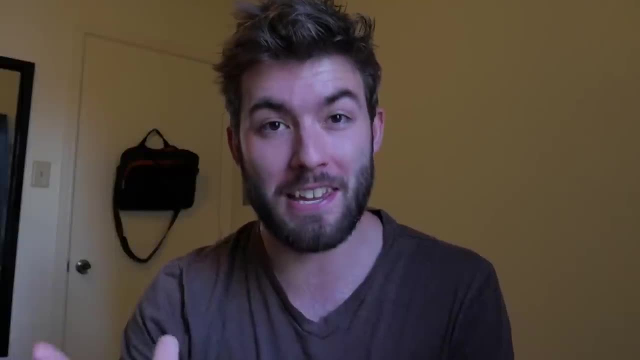 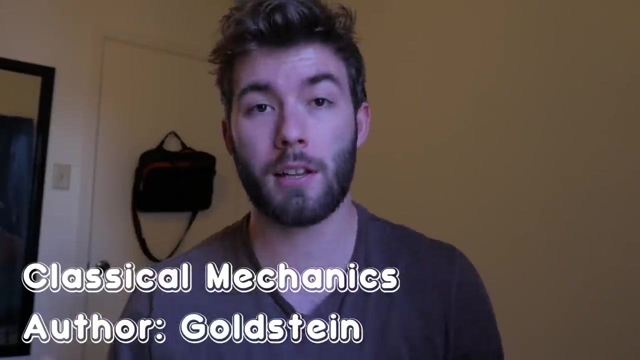 and also I will leave a link in the description so that you can see the PDF version of this book for free. Now, last but not least, is Classical Mechanics, which I've been using the Goldstein book for, and unfortunately I don't have my physical copy of the book yet. 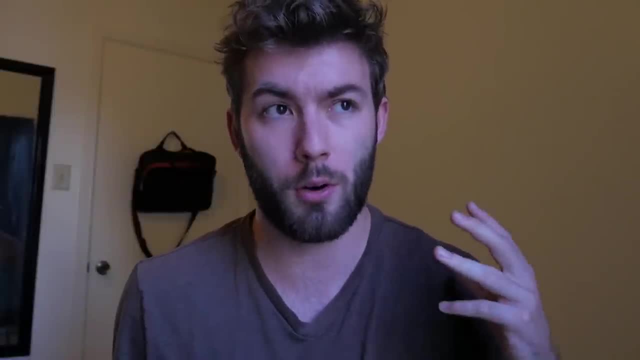 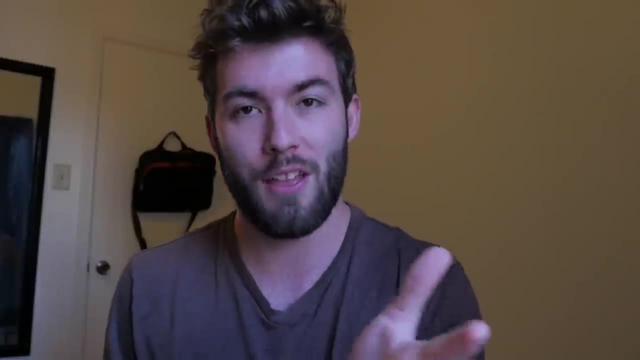 Amazon has been very slow at delivering that to me, so I've been going online and using a PDF version until now. Uh, so, spoiler alert, towards the end of this section, I'm also going to give you the link to that textbook as well. 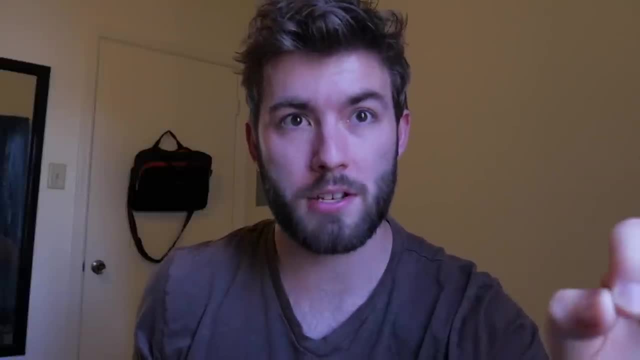 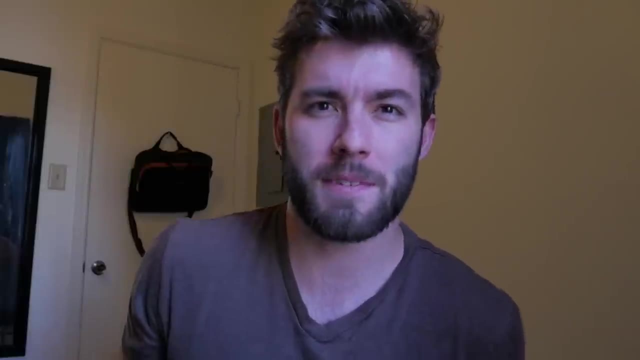 Out of the three textbooks, this is the one that really feels like a graduate physics textbook. I mean, chapter one is Lagrangian's. When I took undergraduate classes, I took the first one and then I took the second one. So in terms of Classical Mechanics, it took probably two-thirds of the semester until we got to Lagrangian Mechanics.